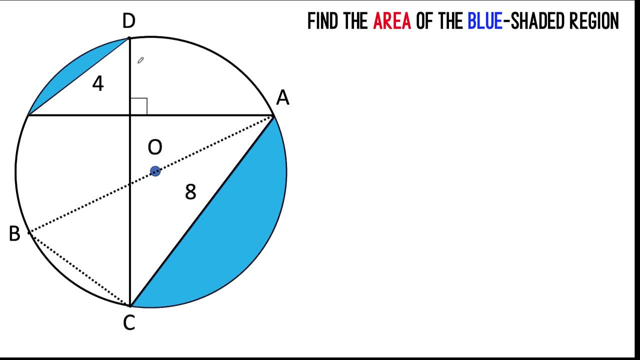 BC. Then let's label the other parts. Let's call this point D and this point as point E. Now what can we say about AB Segment AB is a diameter. That means this line segment divides the circle into two semicircles. So BEA is a semicircle that subtends 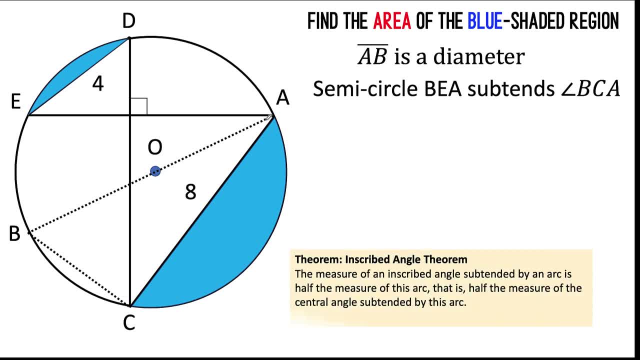 angle BCA And recalling our inscribed angle theorem, the measure of the inscribed angle subtended by the arc is half the measure of this arc. In other words, the measure of this angle here is one half. whatever is the measure of this arc that subtends this angle here? And knowing 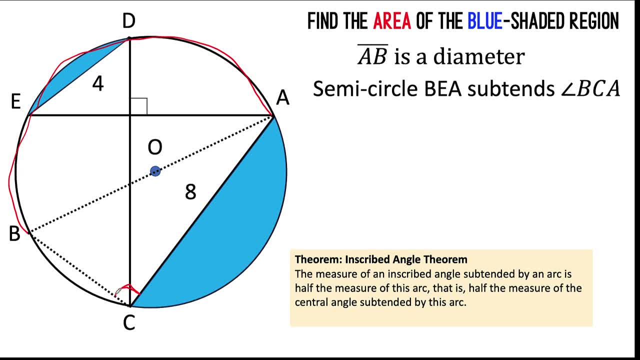 that this is a semicircle, then it follows that the measure of angle BCA must be 90 degrees, Because this angle is one half 180 degrees, which is the measure of a semicircle. Let's call this angle here as angle alpha and let's call this angle here as angle beta. If the angle here is: 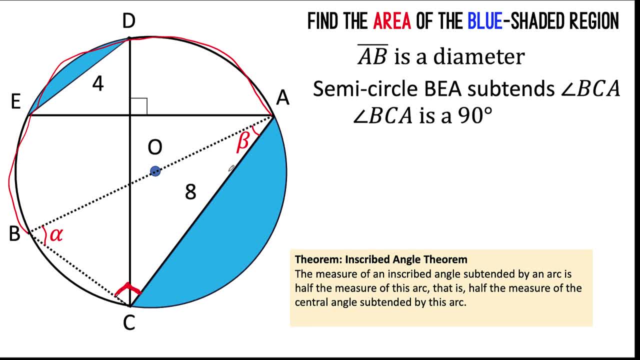 90 degrees. and since the sum of the interior angles of a triangle is 180 degrees, then the sum of alpha plus beta must be 90 degrees. In other words, alpha and beta are complementary angles. Next let's connect point D to point A and let's look at this triangle. Notice that angle ABC. 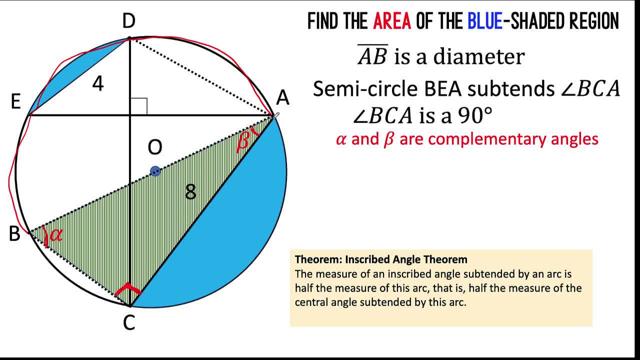 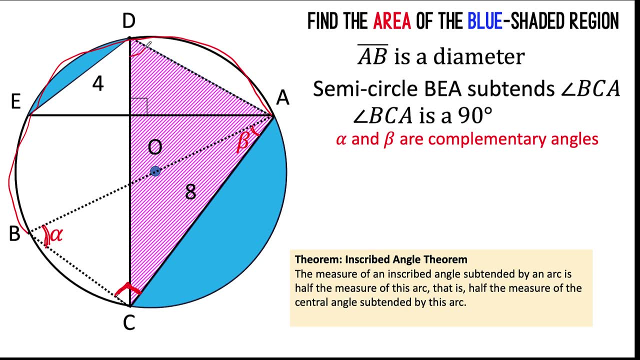 is an inscribed angle subtended by arc AC. This means that the measure of alpha is one half the measure of arc AC. Now let's look at this triangle here, also Triangle CDA. Notice that this inscribed angle here is also subtended by the same arc. 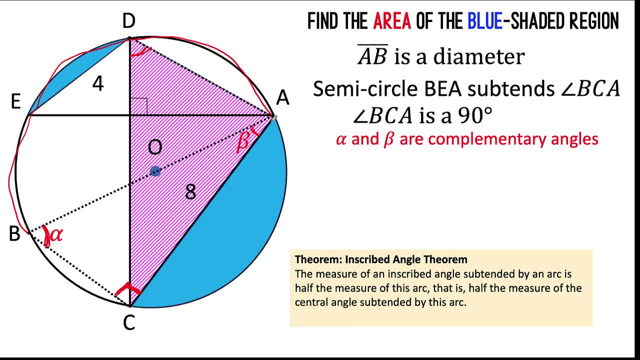 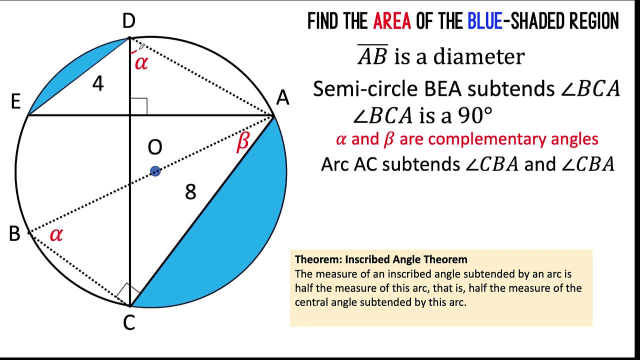 So since these two angles are subtended by the same arc AC, and if the measurement of the first angle is alpha, this angle here must also be alpha. They have the same measurement because they are subtended by the same arc AC. Notice now that we have here alpha and we have here a right angle. 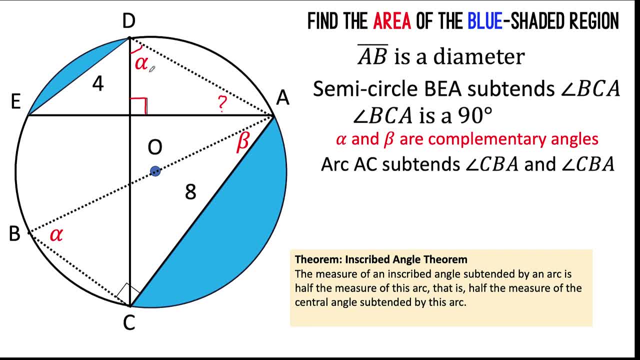 That means whatever is the angle here plus alpha, they must be complementary angles because the sum of the interior angles of a triangle is in the same arc AC. Let's look at this triangle here also, triangle is 180 degrees and we already have here a 90 degree angle. And we said that alpha and beta. 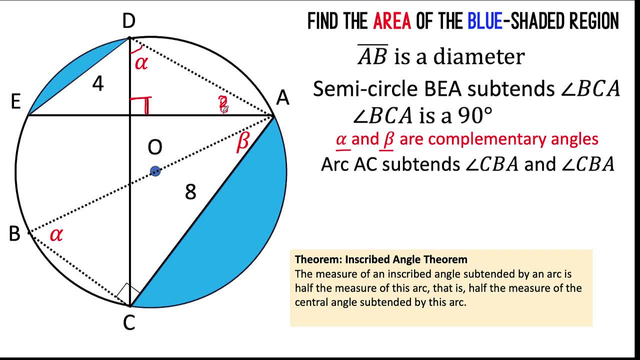 are complementary angles, So the angle here must be beta, So let's label it as beta. You have here beta, and that interior angle intercepted this arc ED. You have also here beta, and the same interior angle also intercepted this arc BC. That means this blue shaded region here must be identical. 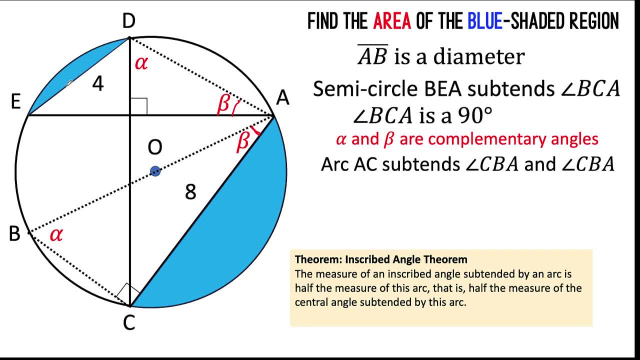 with the region here, And so we can move this blue shaded region here, so that we can just focus on this part here, which is located in one side of this semicircle below. If it was four units here, then this must also be four units, because these two regions are identical. Now, at this point, we 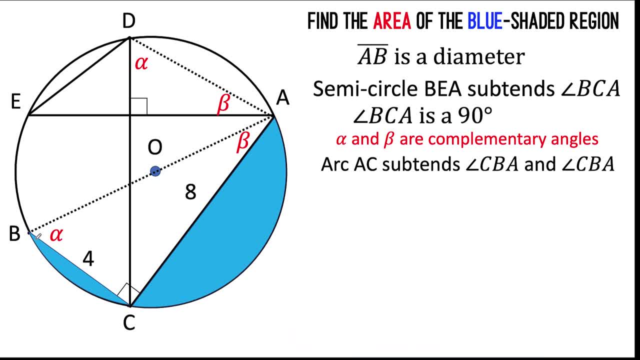 are now ready to find the measurement of the arc BC. So let's go ahead and find the measurement of the arc BC. So let's go ahead and find the measurement of the arc BC. So let's go ahead. and of the diameter, because you have here a right triangle ABC From the Pythagorean formula, the 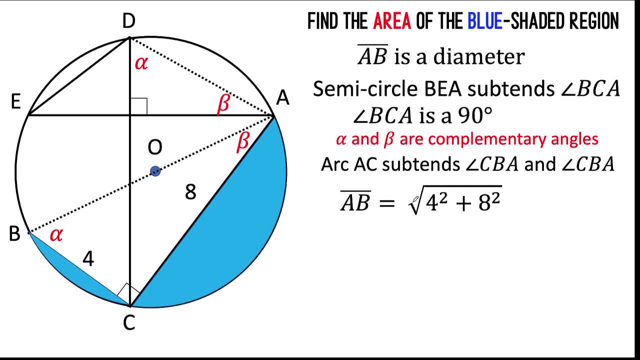 length of our diameter AB is equal to the square root of the sum of the squares of the two shorter sides. So we have here 4 squared plus 8 squared. So solving for the length of segment AB, 4 squared is 16,, 8 squared is 64, and 16 plus 64 is 80. So the length of segment AB is square root of 80, or 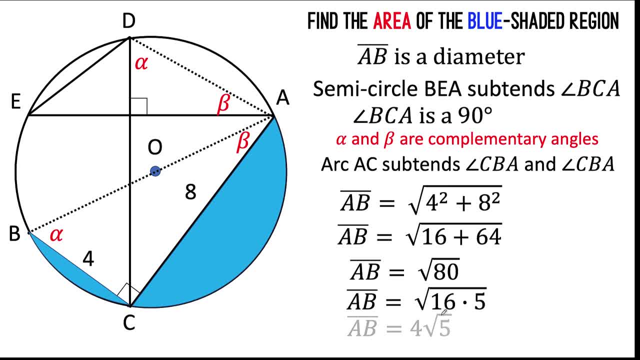 80 is 16 times 4.. So we have here 4 squared plus 8 squared. So solving for the length of segment AB is: 4 squared plus 8 squared is 5.. The square root of 16 is 4, and cap is square root of 5.. So the 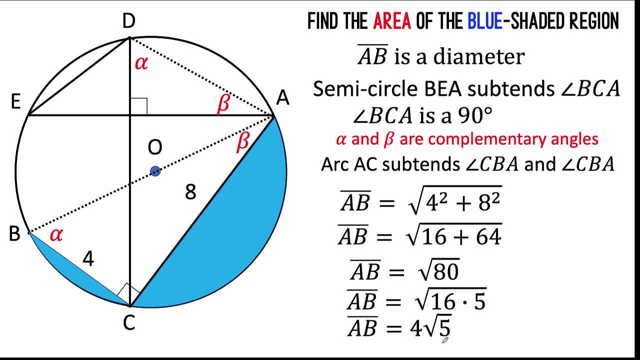 length of our diameter is 4 squared of 5, which means that the radius is one half 4 squared of 5.. So the radius is 2 squared of 5.. Now that we already know what's the length of the radius, 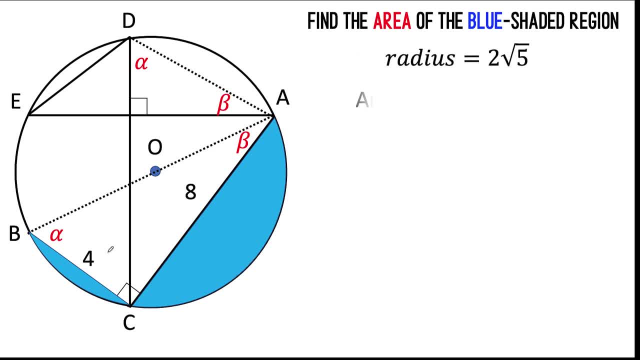 then we can now find the area of the semicircle. The area of the semicircle is one half the area of a circle, So it's one half pi r squared. We know that r is 2 squared of 5, so substitute that in the formula We now have here. the area of the semicircle, s is equal to.